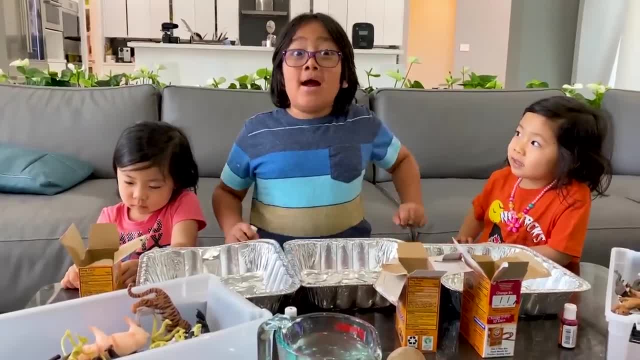 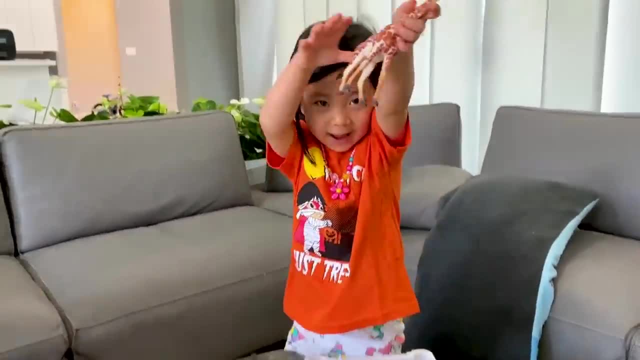 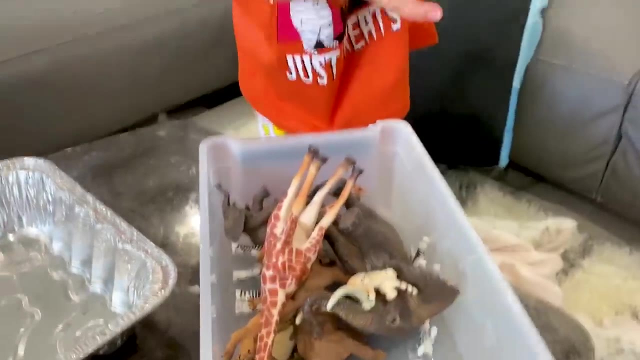 Hi guys, Today we're doing a science experiment where we hide surprise toys. I think I'm going to die. I want to go home with them now. Welcome to Ryan's World. Yes, so we have all the leftover toys here. Scary, Scary Where we're going. 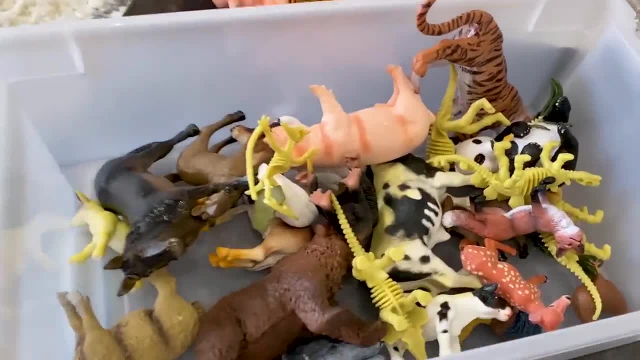 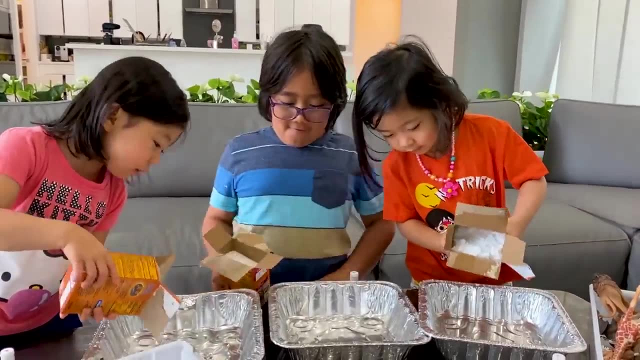 Here, Ah, Piggies, Yeah, so we have all these surprise toys here. We're going to hide. First, we're going to put in baking soda. All of them, All of them, All of them, The whole thing, The whole thing, yeah. 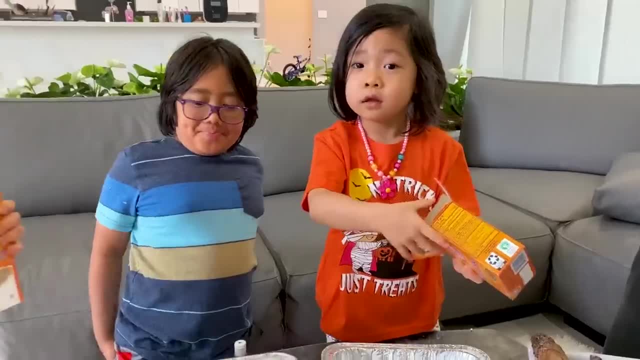 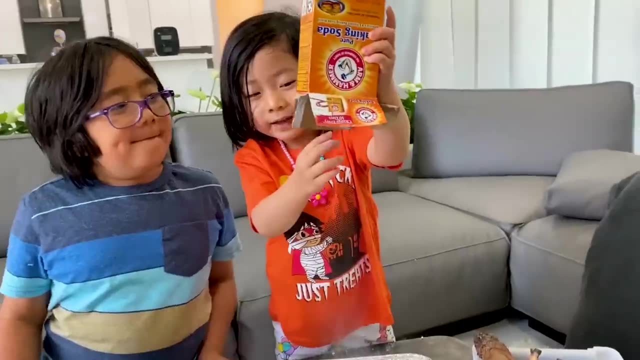 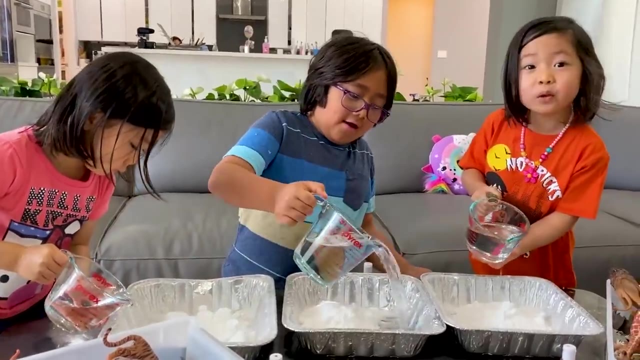 Whoa, Do you have a lot? Yes, Emma Woo, It looks like a big coffin. Yeah, It looks like snow. Looks like snow. Next let's add in water. Now we're going to be doing all of it, All of it, yeah. 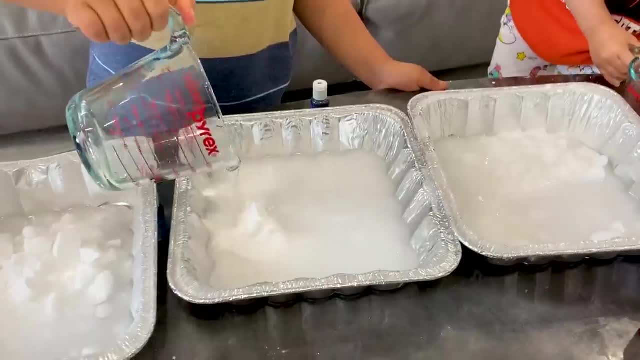 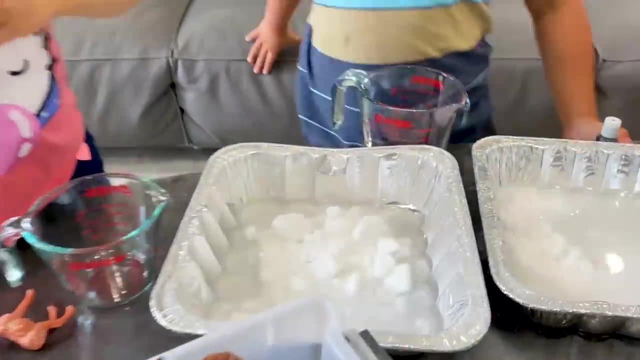 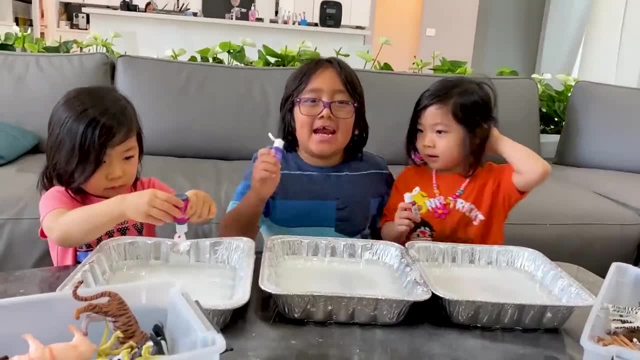 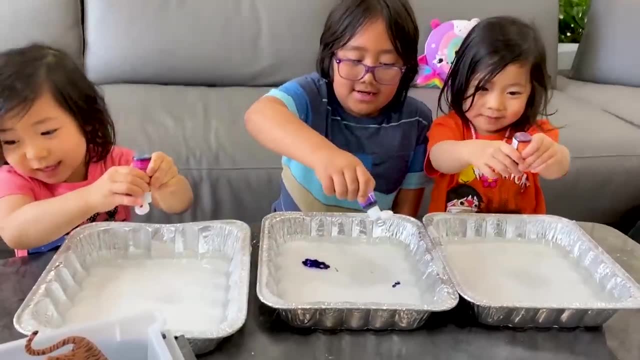 Yeah, Next, add food coloring, and I'm going to use purple, I'm going to use pink. I'm going to use pink, And I don't know where all of them are. Like a peach, I add one drop. Next up, let's add the pink. 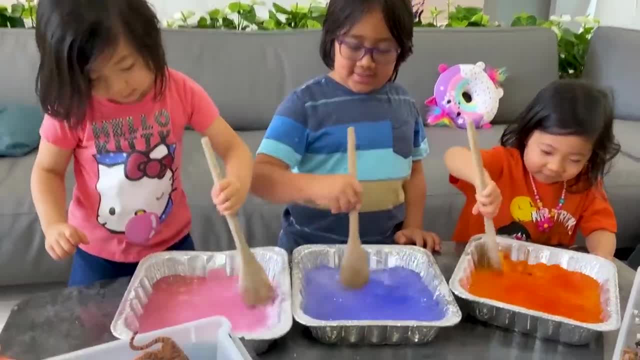 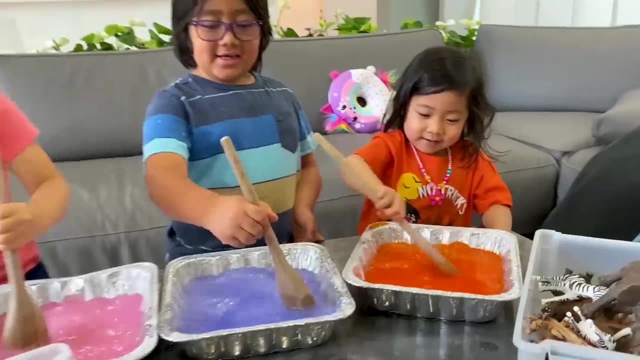 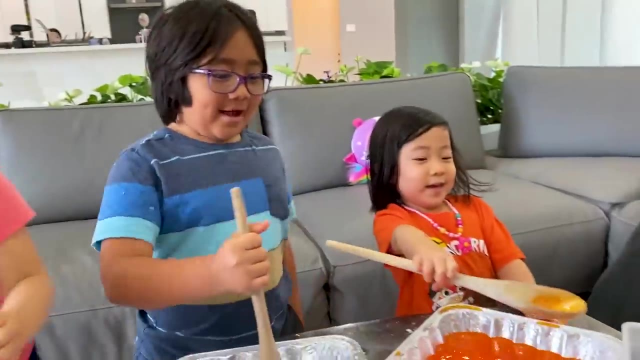 Add the pink, then Mine looks like a piggy, Mine looks very purpley. Mine looks bubbly, Mine looks purpley, Mine looks bubbly, Mine looks purpley, Mine looks bubbly, bubbly, bubbly. Whoa, another witch. 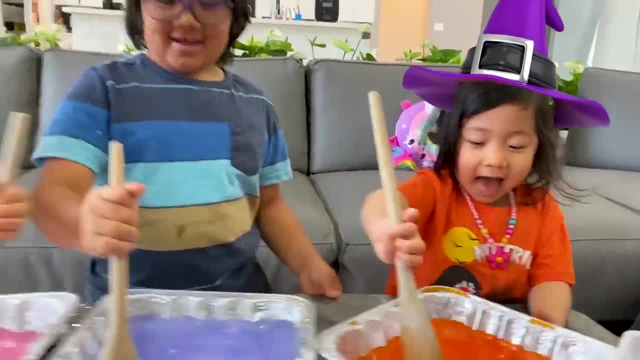 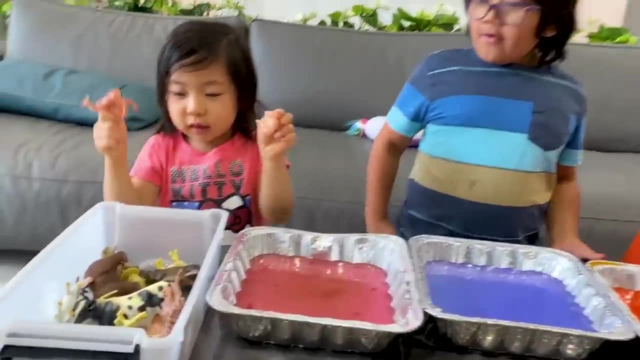 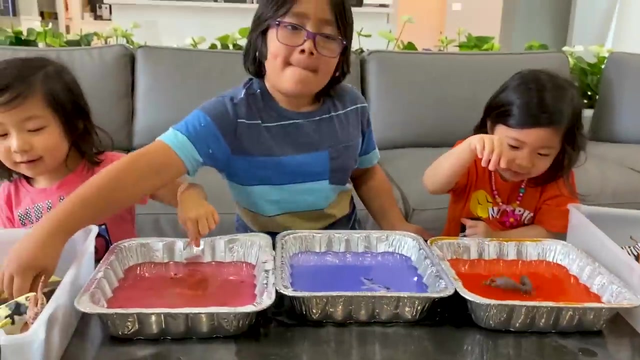 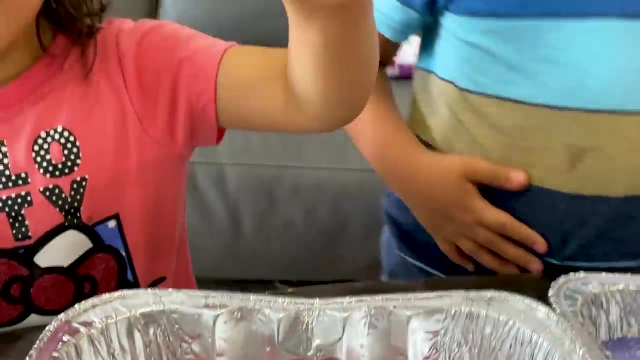 I like your laugh that much. There you go, Put some presents, Yeah, anything you want. Ryan picked a cat, Baby, elephant And the bear And a lot, Oh, and a dinosaur. No, it's fine, You can put it. Try, Saratop. 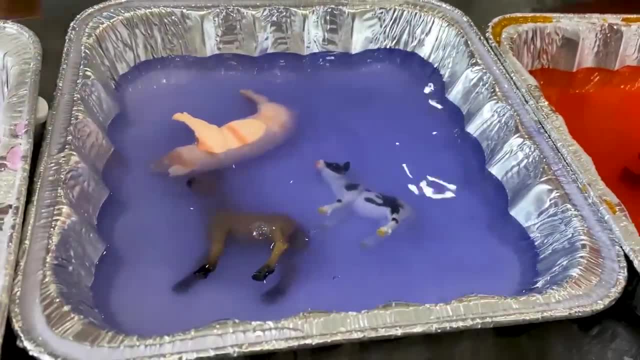 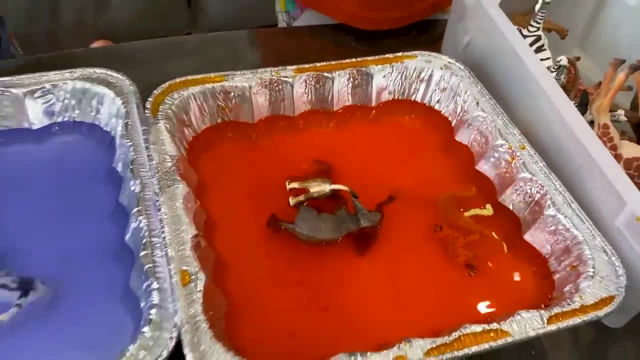 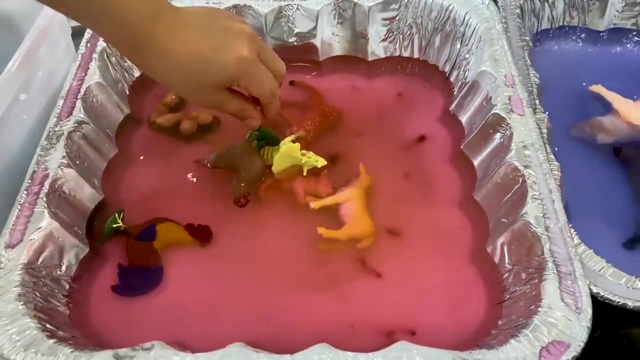 I'm putting in a horse. Okay, so just add in a couple. What about this one? Sure, Okay, Whoa, chicken And rooster. Are you guys done? Yeah, I want one more. Okay, Emma, Can I have one more? 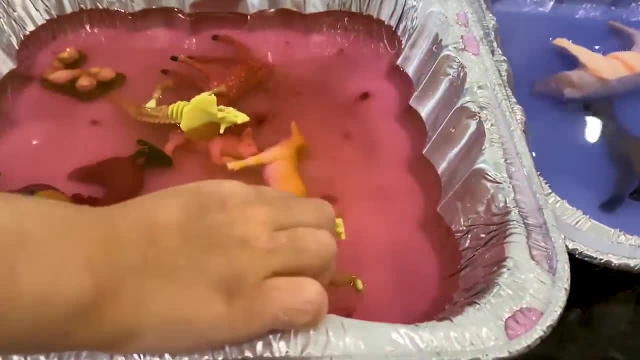 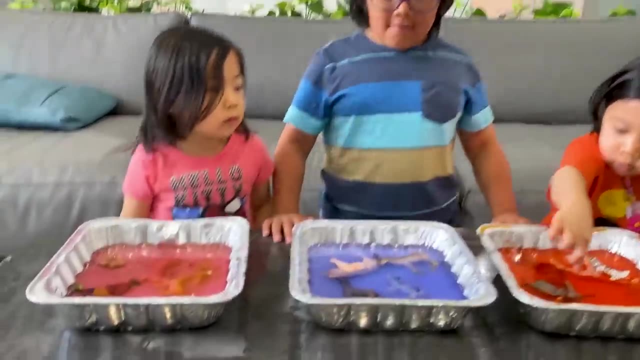 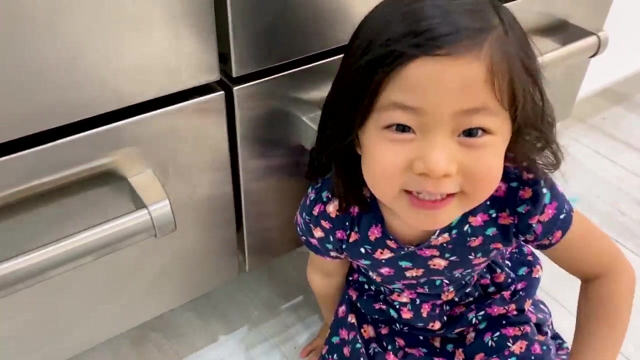 Okay, Mommy's a bear, Mr Outer Bear. Oh, another dinosaur. Now let's put it in the freezer, Alright. so Mommy's gonna do that Freezer time. Okay, we're gonna freeze it, Alright. I think it's ready. 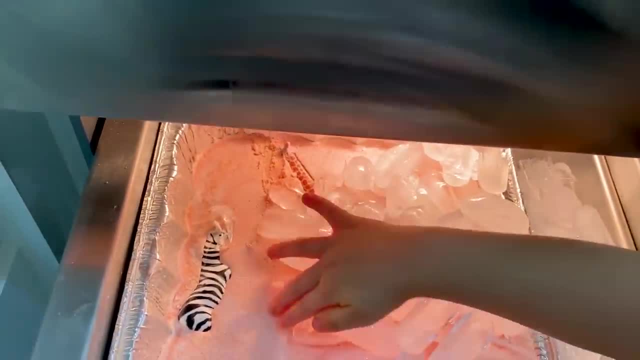 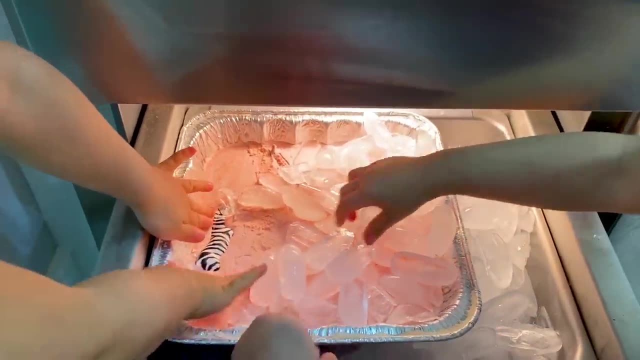 Okay, let's see. Whoa, Wow, What food is this one? Oh, this one has ice on it, because I accidentally put it in the ice tray. Is it cake, Ryan? I don't remember. Alright, let's take it out, guys. 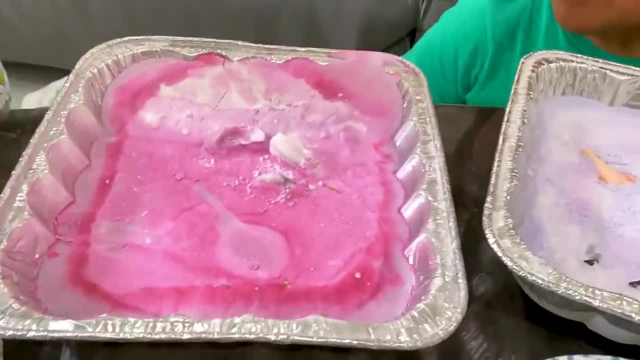 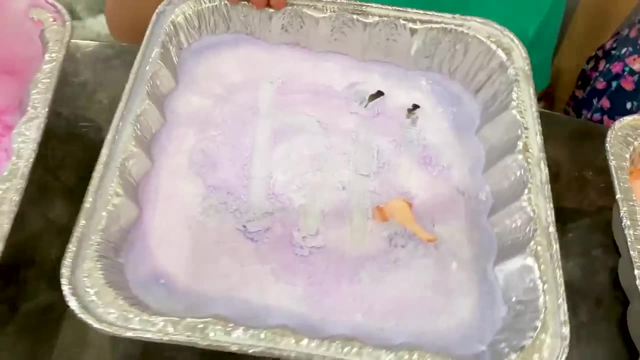 Okay, guys. So now that we got it out of the freezer, that's what it looks like. Some of them have ice in it, but it's okay. Oh, Ryan, did Ryan put high with his hand there? Now, these are vinegar, so what you're gonna do is: 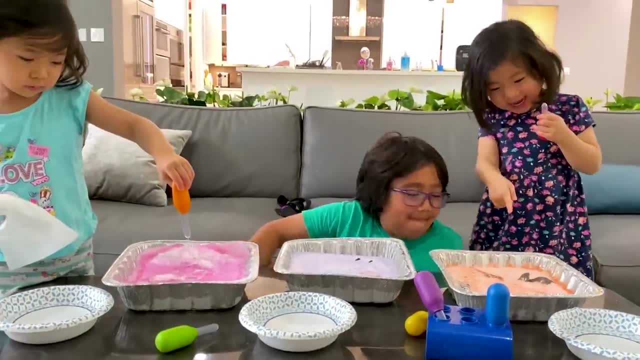 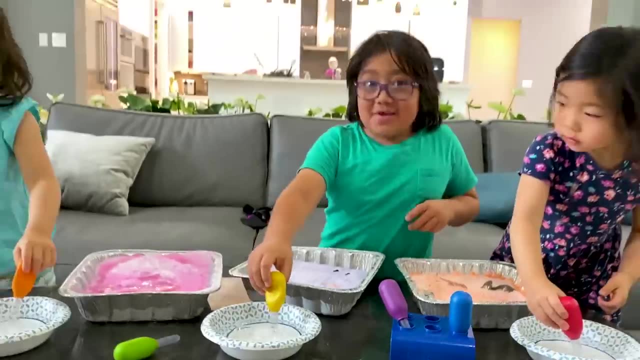 you're gonna put vinegar into your baking soda. I see ice, Oh Yeah. so what we're trying to do is rescue the animals that we put in there. Rescue the animals. Yes, that's the goal: Rescue the animals. So why do we put the animals there? 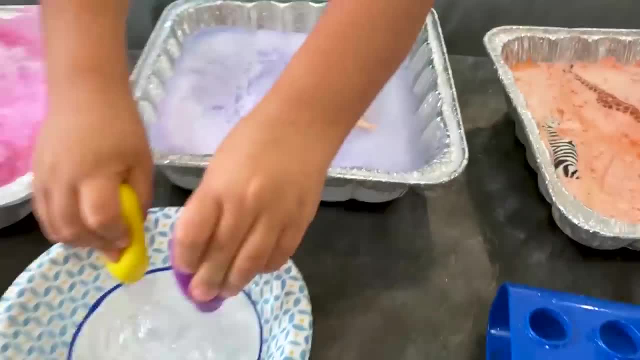 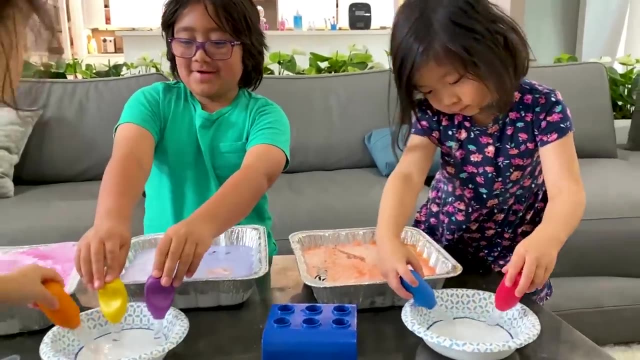 They're having a fun bath. I'm trying to get this one animal. What was that? Did you guys see it? I don't know what it is. It looks like a pig or something. Now it's Kevin. Oh, I'm saving both of them. 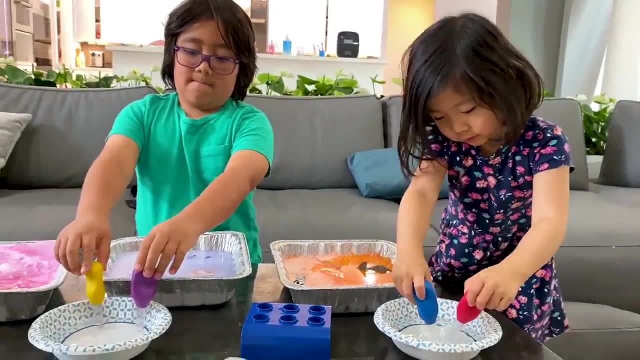 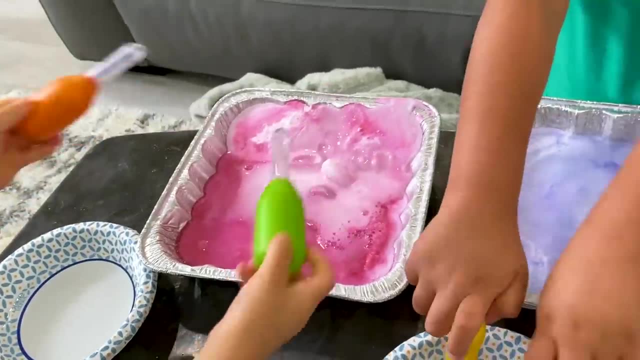 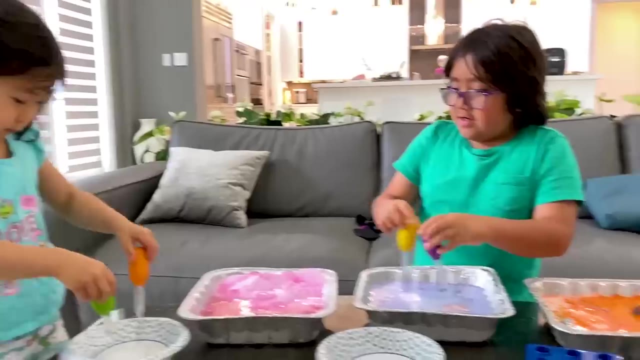 I would save mine. I have a lot, I know Whee Whoa. Good job K. Do we have to save the animals? Yeah, save the animals. But why are they having a bath? They're having a bath, Yeah. 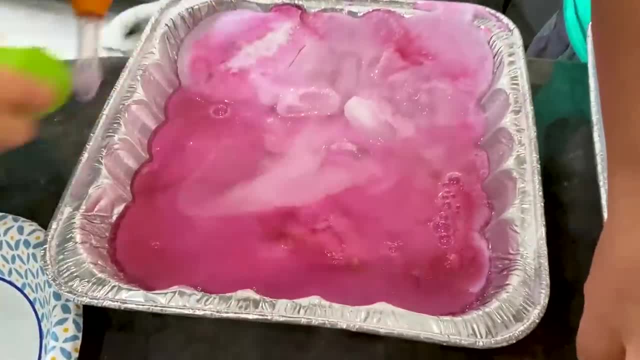 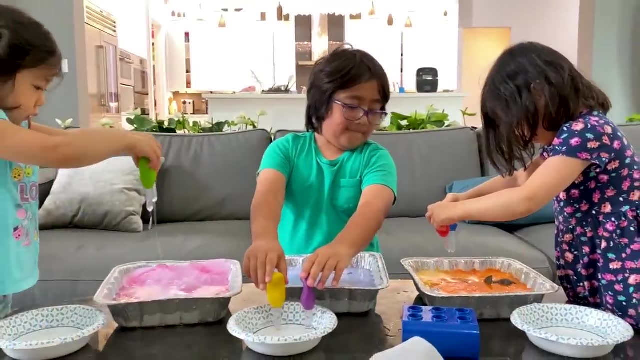 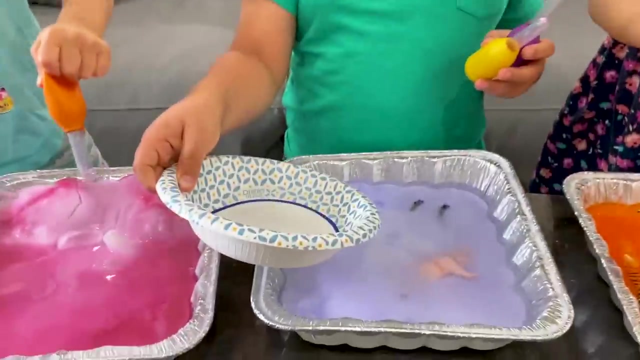 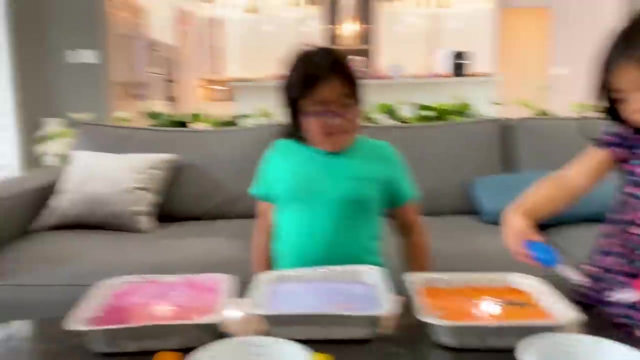 Why, Whoa What Everybody helping each other. How nice Looks good, Emma. Yeah, I'm gonna put the whole thing in because it's not going that fast. Me too. Whoa, You wanna do that too? Not yet. 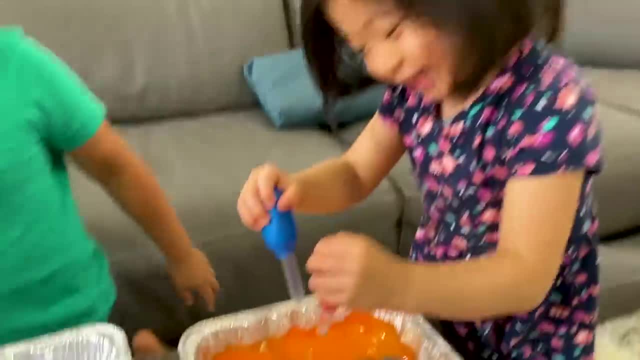 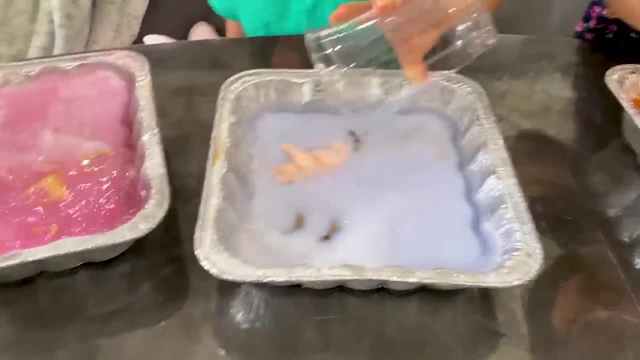 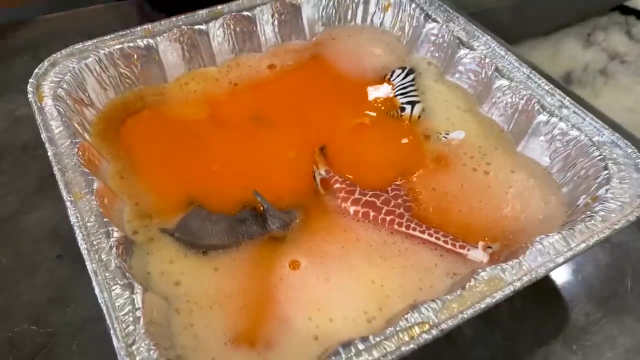 We need way more. Yeah, Emma, All right, so now I'm just gonna give them a cup of vinegar. Whoa, look at it- bubbles. Look at it, bubbling, It's bubbling. Yeah, Can we save the animals? 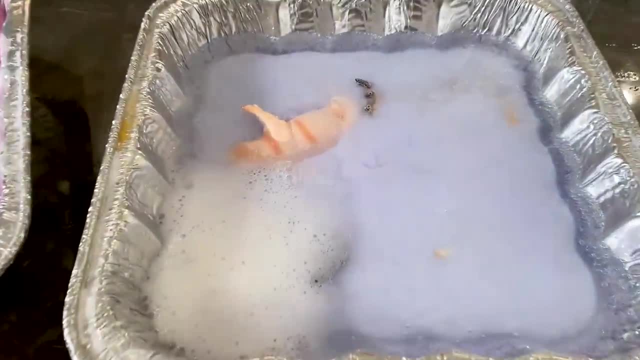 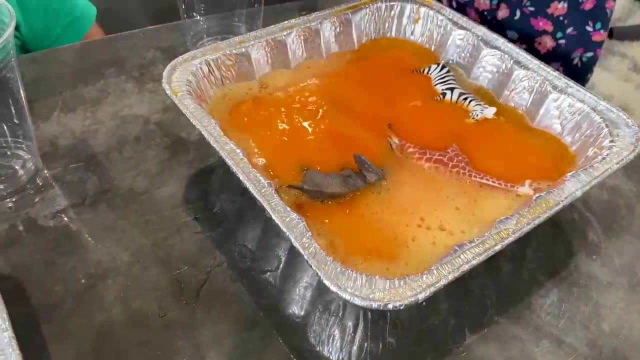 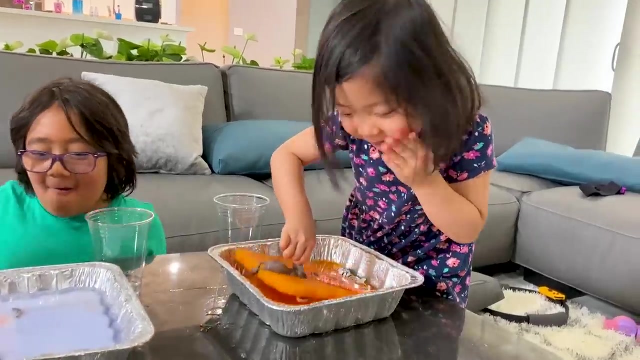 Yeah, Can we save the animals? I want that animal, Oh almost, Can you take it out? Let's see if Emma can take it out. Almost, I cannot, Ryan, Not yet. Whoa, So close, Can you suck into that one? 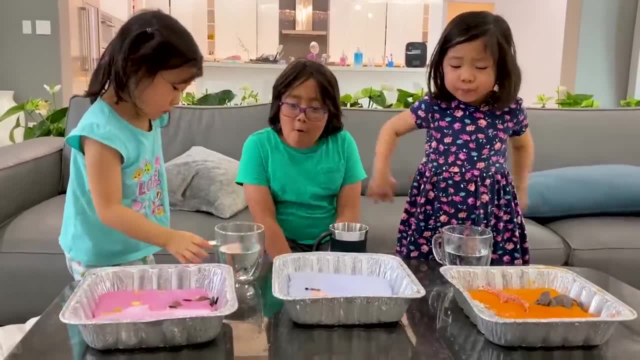 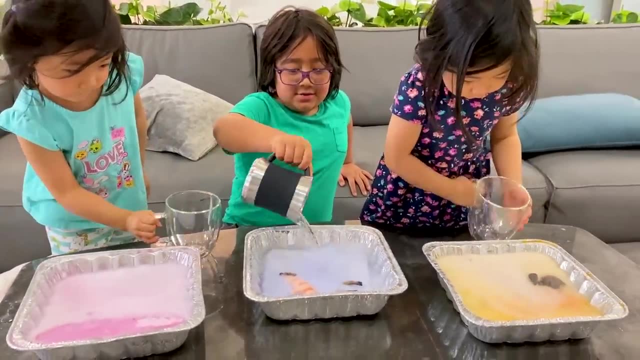 The animal's on the other side. Okay, guys, we are so close, We're gonna try one more time. Can we rescue the animal? Oh, that water probably works a lot more. Yes, we actually warmed up a water. This is a fun video because 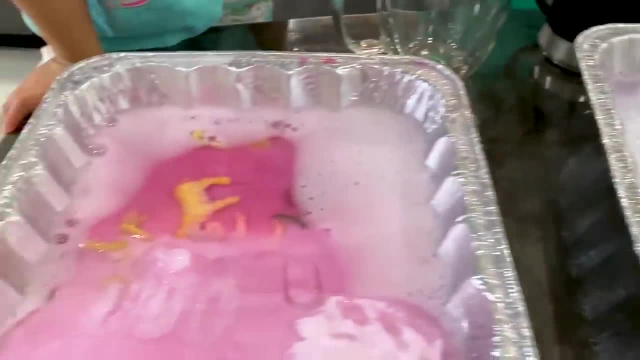 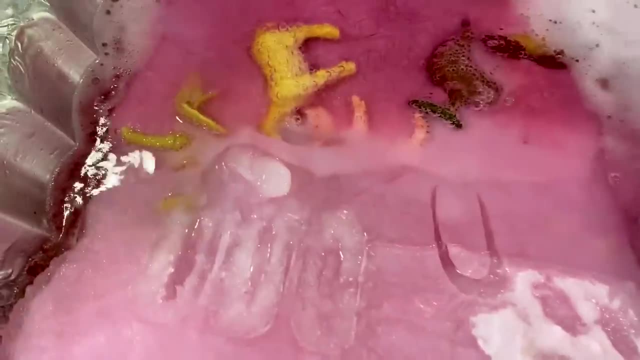 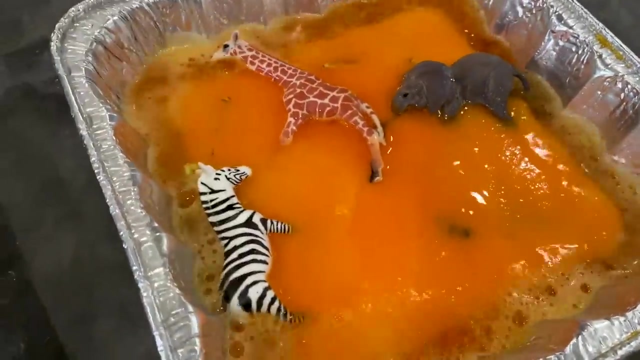 the kids can help each other figure out how to rescue the animals. Mommy, Yeah, almost So close. You can see the animals here So close. Ryan's so close. Look, it's moving, I'm gonna get mine out. 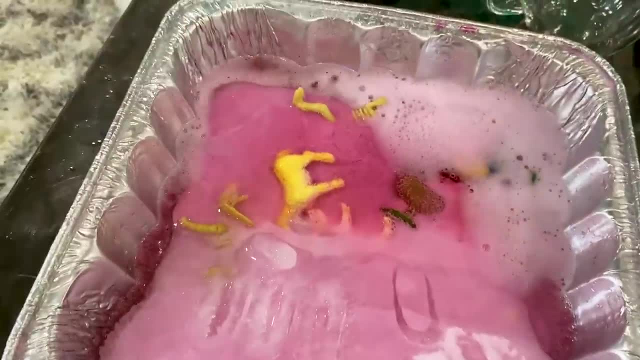 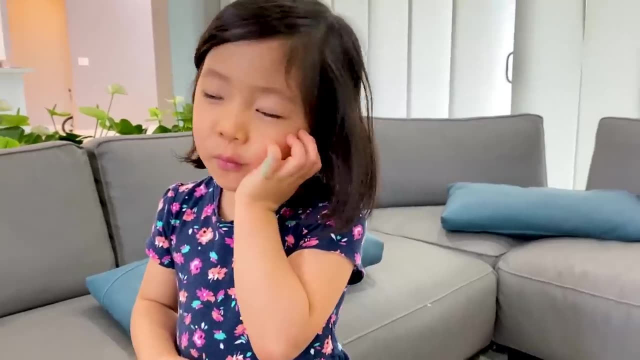 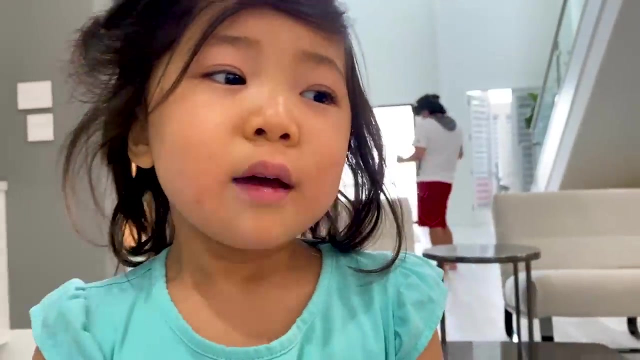 Look, I'm gonna get mine out. I know That's the point. We gotta figure out how can we rescue the animals. How about we do hammer? Good idea, All right, Strong hammer's for us. Yeah, Good idea, Ryan. 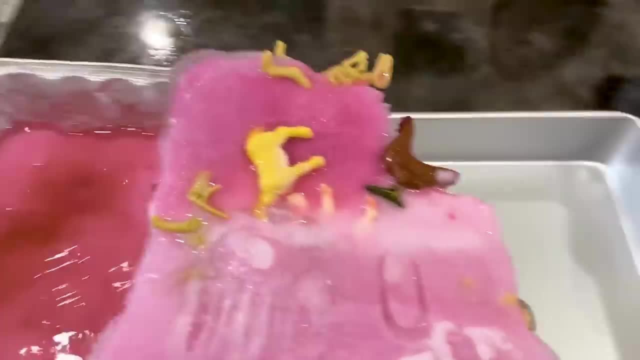 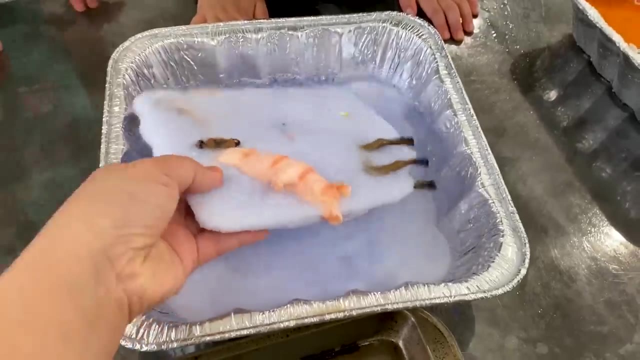 First, Mommy's gonna help put it into a tray so you guys can break it up. Look, We got one. Yay, Good job. Okay, this is Ryan's. I'll take it out for him, And it's almost done. 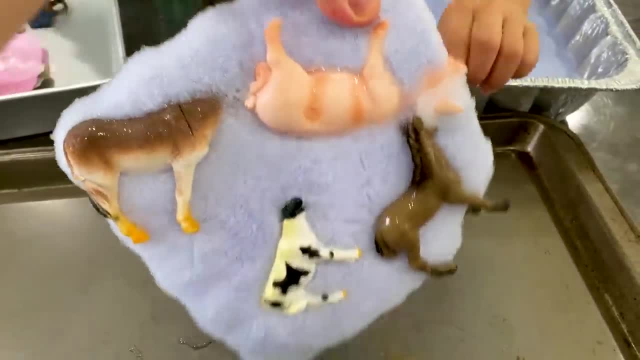 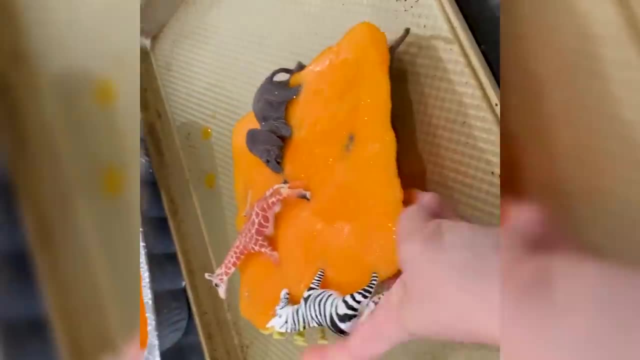 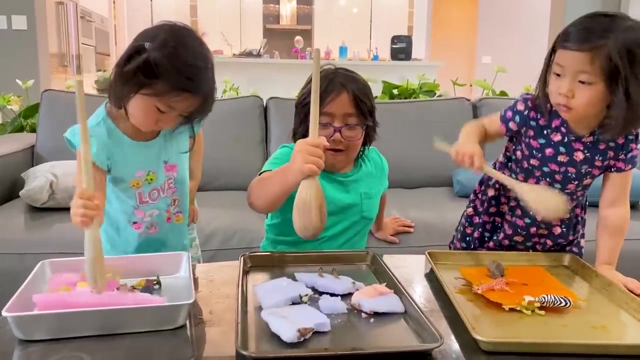 Look, Look at the back side. You guys can see what animals he picked out, And this is Emma's Really really close Her front and back side here. She also picked a dinosaur. We actually don't have a hammer, So I'm giving her a spoon. 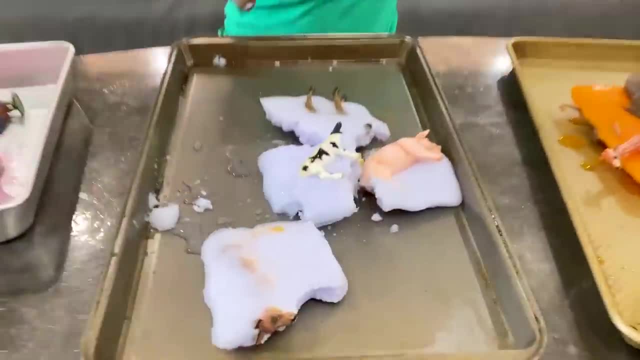 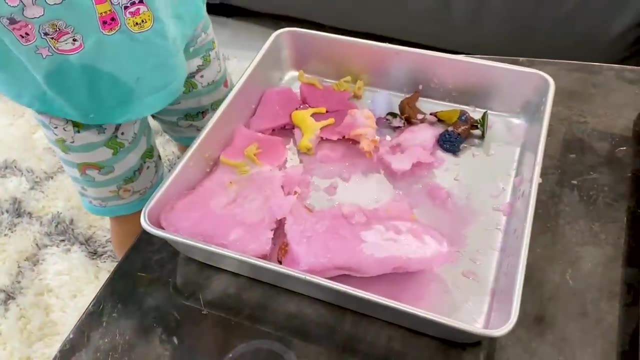 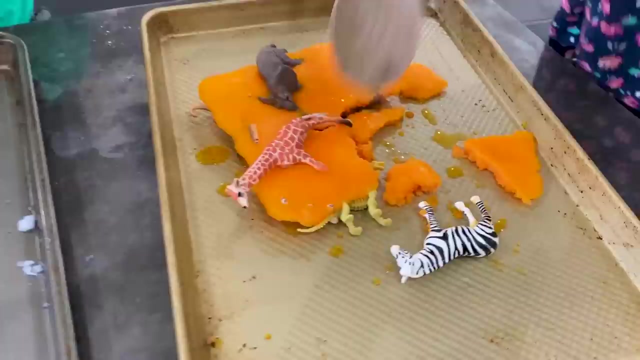 Whoa, Ryan, Good job. Whoa, Whoa, Whoa. okay, This is a very messy experiment. I got one out. I think that's it. You rescued the zebra. I'm gonna rescue the pig. Is this really rescuing? 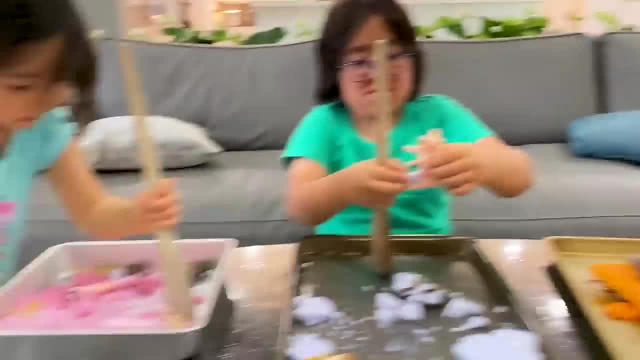 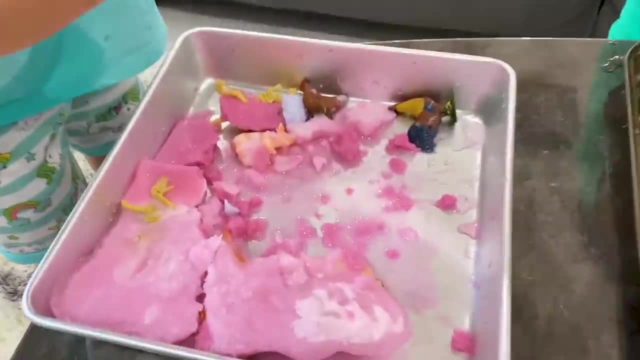 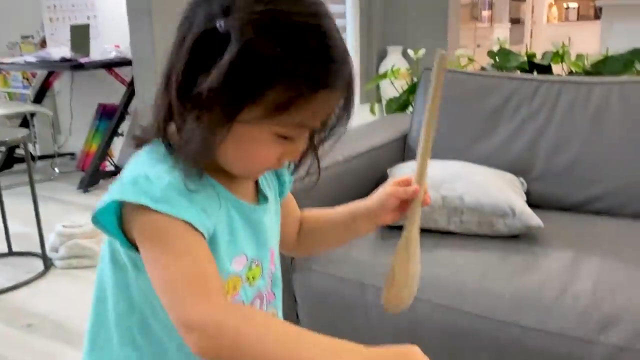 What about you, Kay? Did you, You did? Did you rescue anybody? Wow, Almost done. Whoa, Baby giraffe. Good job, Look, I got the pig. You did Ryan, Nice, Just one more: The horse. 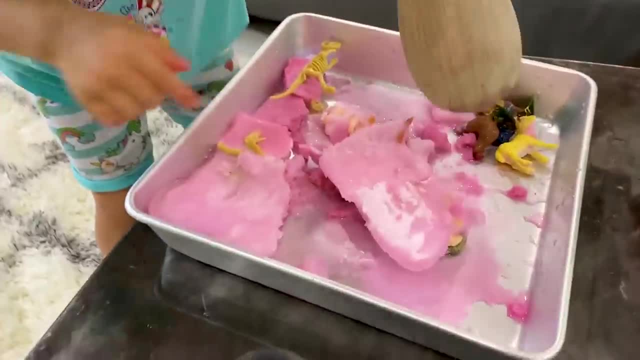 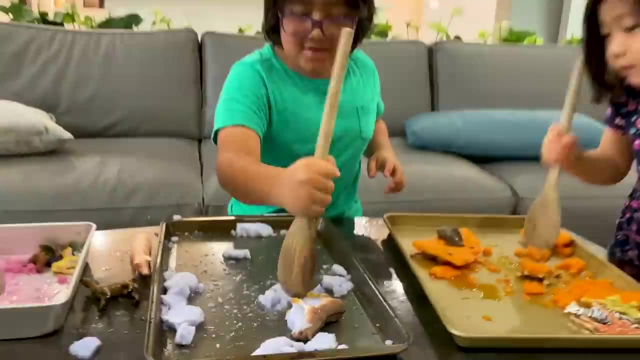 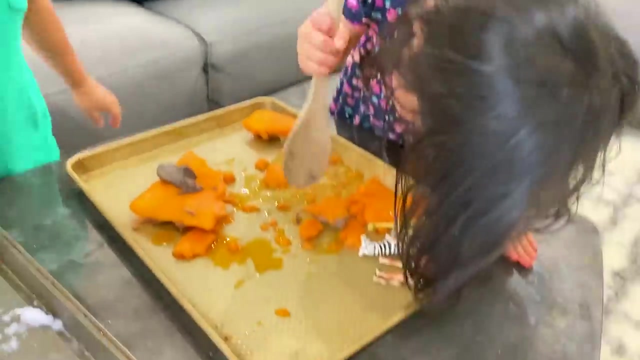 I got the baby, I got the horse. Nice, Oh, one more. What is that? Is that a donkey? I forgot, It's a hyena, A hyena, Whoa. I think this is a baby tiger. 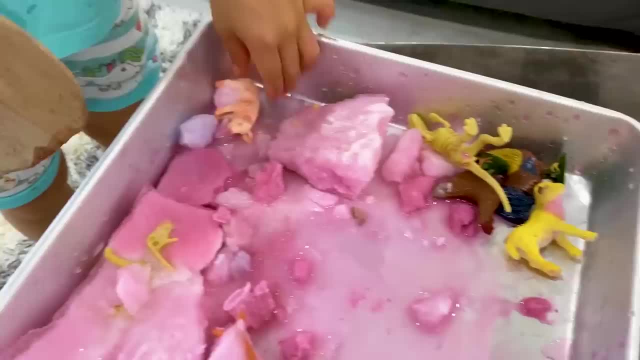 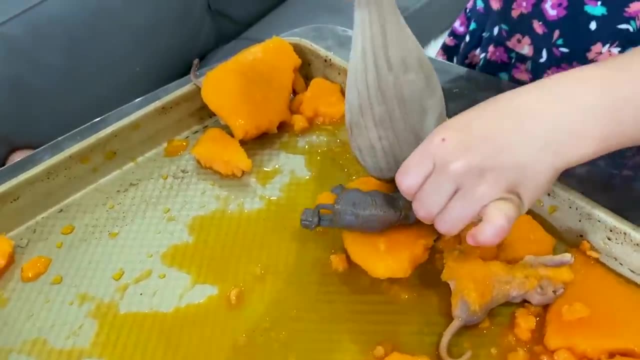 You got a baby tiger. Yeah, Wow, Kay's almost done. Look, She just needed to rescue the piggy And then there's one giant dinosaur. Huh, What is that Elephant? I think it's a mommy elephant for the baby. 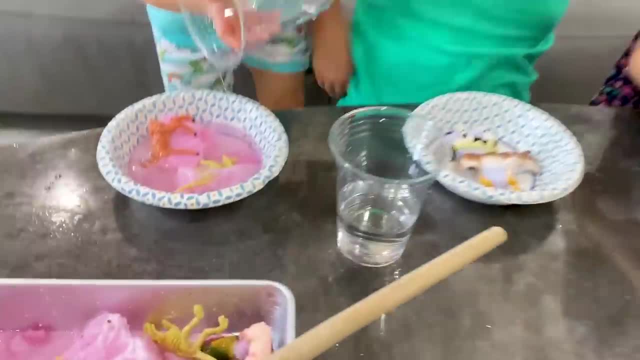 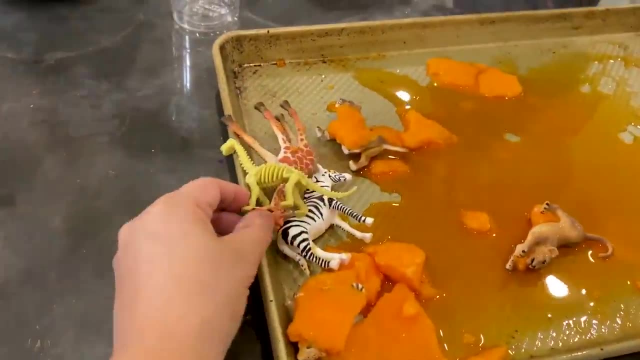 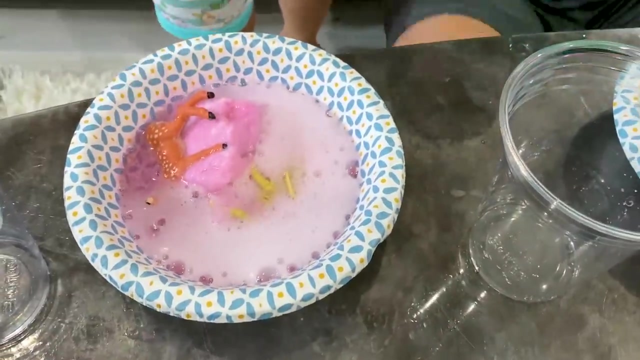 Whoa, Almost done All right, So we just have a few more animals here to rescue. Okay, Yeah, They rescued pretty much all the animals already, Except for these. Oh, look, It's going. You see the bubbles? 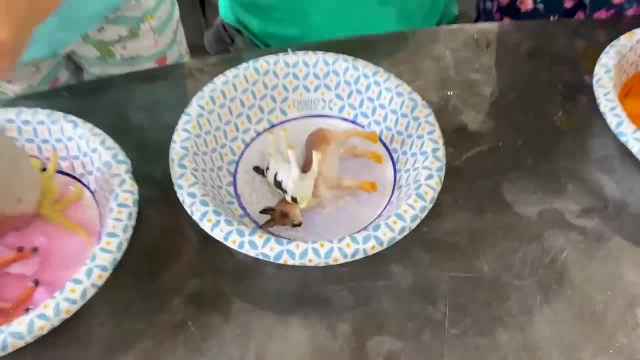 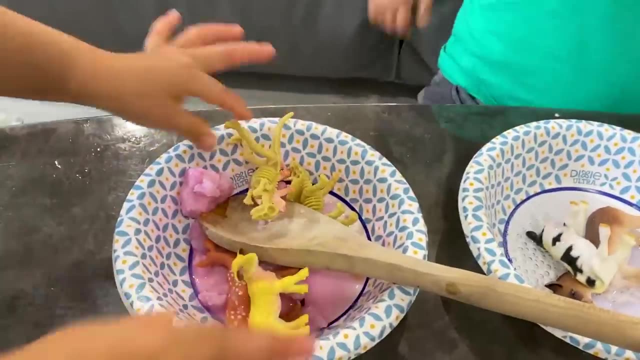 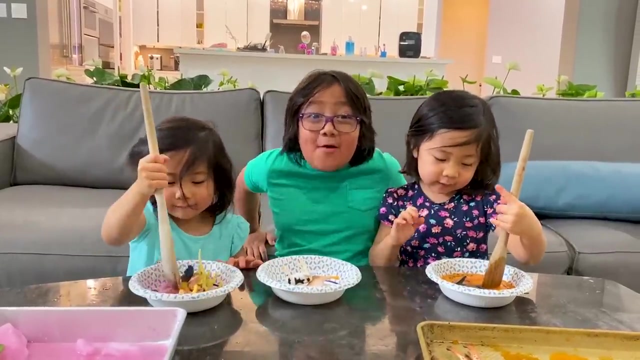 Look, We rescued all the rest of the animals. Look It's out. So Emma's almost done with hers. Yeah, Good job, Looks like soup. Bye, guys, Thank you for watching our video on rescuing animals. Bye. 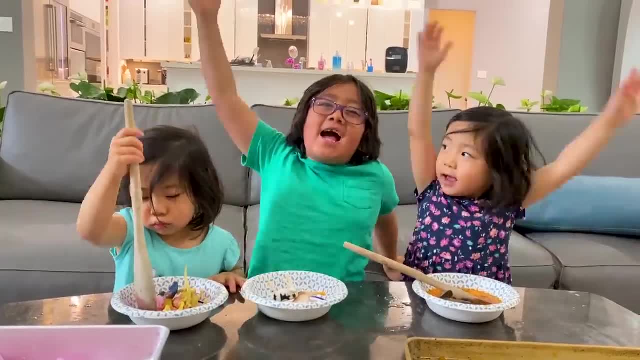 Remember always, stay happy and rise up. Bye.